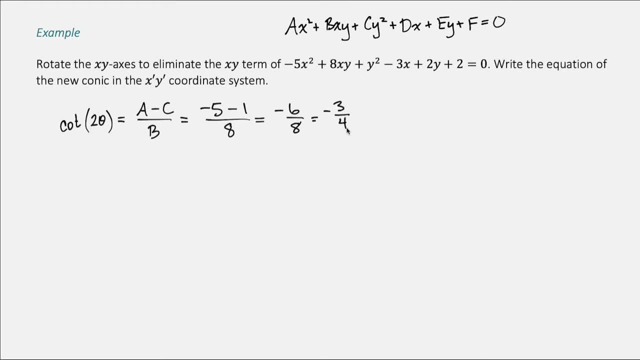 Now we have cotangent of 2 theta equals negative 3 fourths. When we're trying to write the new equation in the new x prime, y prime coordinate system, we don't actually need to know what the angle theta is. We just need to get this and then we'll need to find the sine and the cosine. 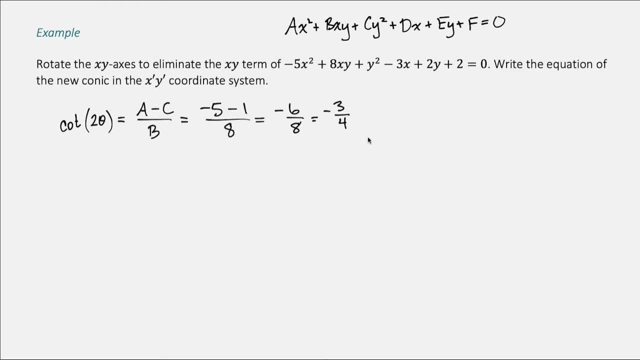 So there's a couple things to do. The first is we're going to kind of draw where the angle 2 theta is, because we have a negative number for our cotangent And this conversion only works when 2 theta is between 0 and 180 degrees. 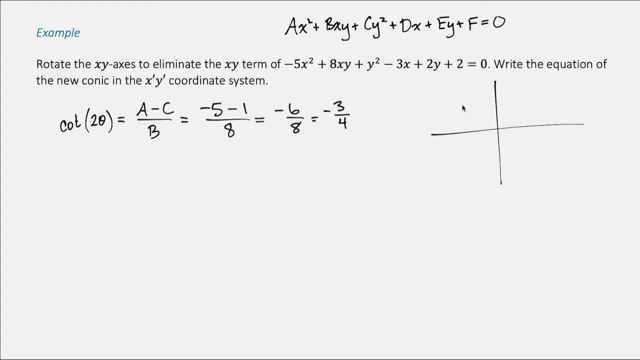 We know that we're going to be in the second quadrant here, since cotangent is negative in the second quadrant. So we have some angle here And if I draw a triangle I can draw any triangle here with that angle of 2 theta. 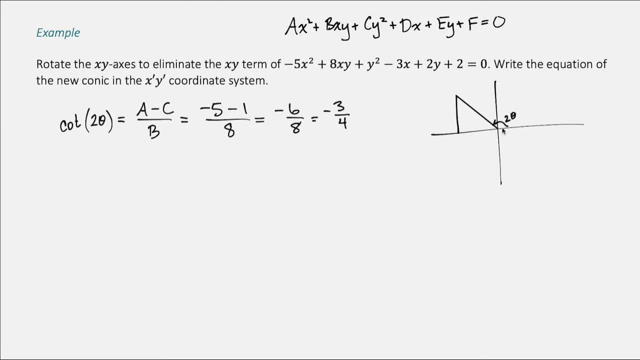 This is 2 theta. here, I know, cotangent is the x over the y, And so I can write that as a negative 3 over 4.. Note that the 3 has to be negative. since I'm in the second quadrant, The 4 has to be positive. 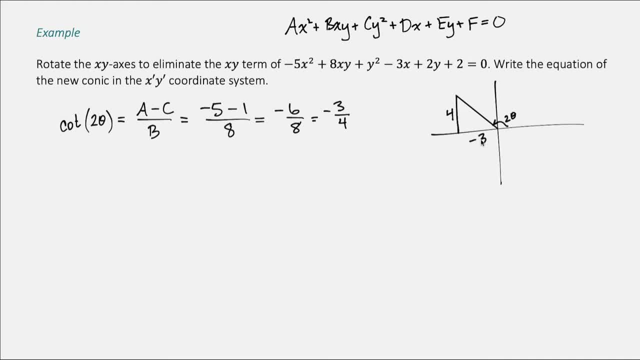 Using those two side lengths. I can use the Pythagorean theorem to get this side length here. That's the classic 3,, 4, 5 triplet Pythagorean triple, So I don't have to do much work there. 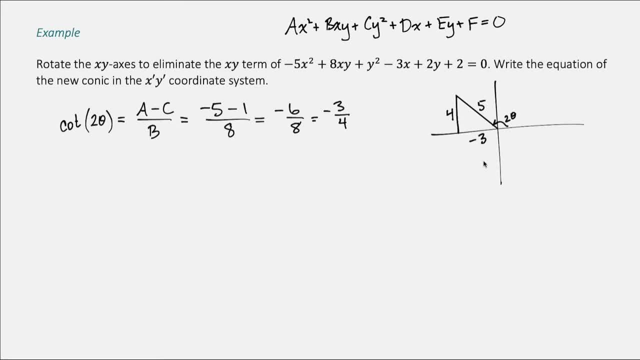 Now that I have that, all of the conversions from the a b, c d to the a, prime b prime, c prime d prime, Those conversions all use the sine of theta and the cosine of theta, And so we need a couple of identities here. 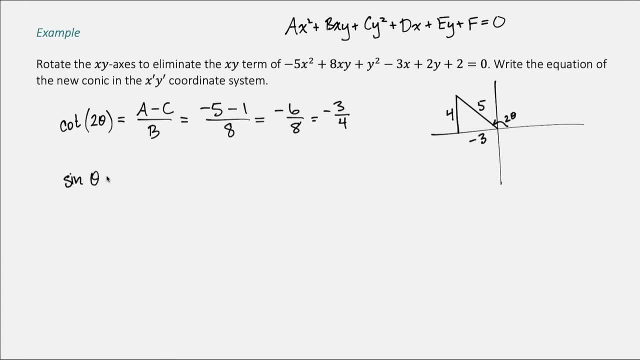 Sine of an angle theta. This just comes directly from. this is actually the half angle identity, but using a theta here You get: sine of theta equals plus or minus the square root of 1 half times 1, minus cosine of 2 theta. 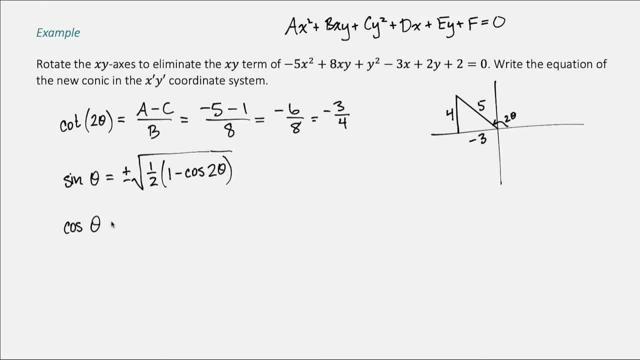 And we have: cosine of theta equals plus or minus the square root of 1 half times 1 plus the cosine of 2 theta. Now, the plus or minus in each of these is simply determined by which quadrant we're in, Whether the sine is positive or negative, and similarly for the cosine. 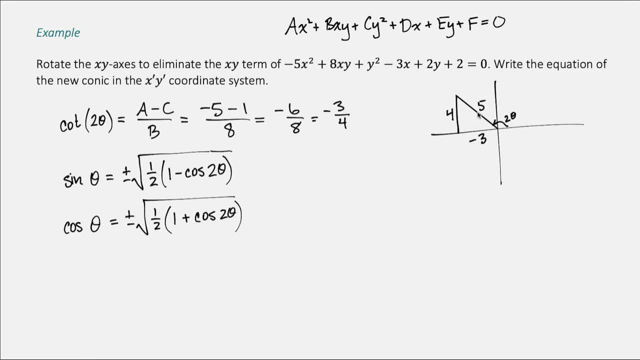 Because 2 theta is in the second quadrant. I know theta is in the first quadrant And that means that both sine and cosine will be positive. So we'll be using the positive in front of each of these square roots. And then cosine of 2 theta is. I can get from this triangle here. 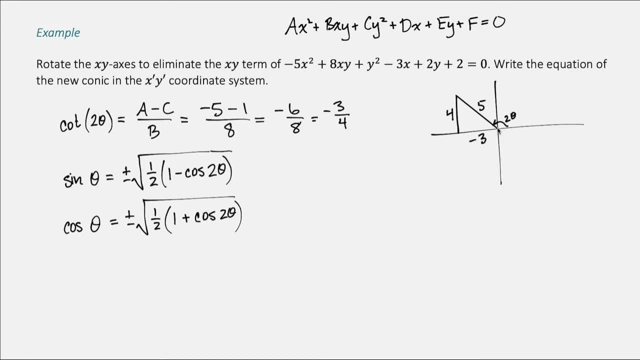 So cosine of 2 theta- here cosine is going to be the adjacent over the hypotenuse, Or x over r, So that's negative 3 fifths. Cosine of 2 theta equals negative 3 fifths, And so now I can go in and find each of these. 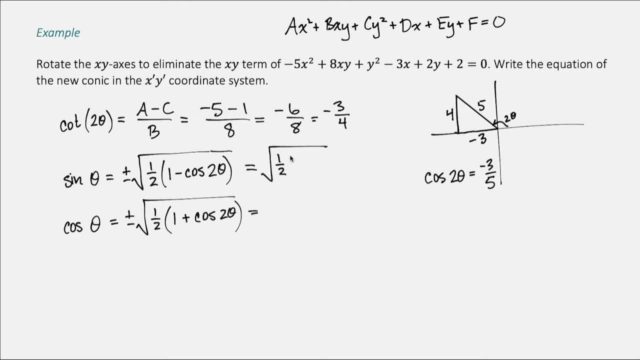 So I have the square root of 1 half times 1 minus negative 3 fifths, Which is 1 plus 3 fifths. And here I have the square root of 1 half times 1 plus negative 3 fifths. 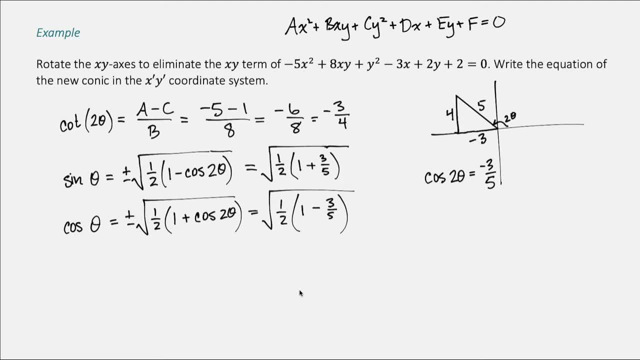 So minus 3 fifths, And then of course, I can simplify each of these. So 1 plus 3 fifths is 8 fifths Times 1 half is 4 fifths. So this is the square root of 4 fifths. 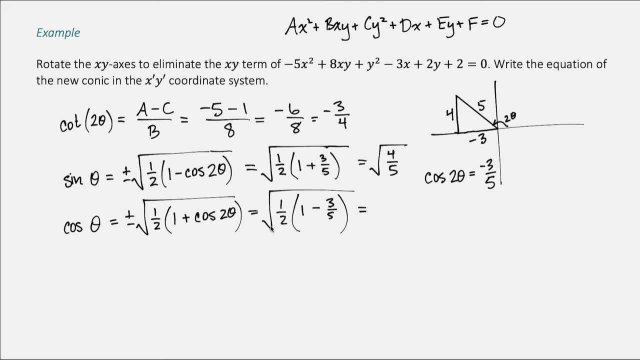 And here 1 minus 3 fifths is 2 fifths Times 1 half is 1 fifth. So this is the square root of 1 fifth. Now I have sine of theta and cosine of theta. I'm ready to go through and find all of my new things. 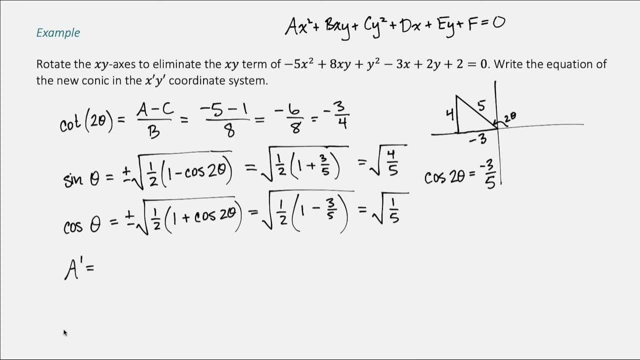 Coefficients, So A prime. The conversion is A times cosine squared of theta Plus B times cosine theta sine theta Plus C sine squared theta. And so now I can go through and plug in everything that I know I have. A is negative 5.. 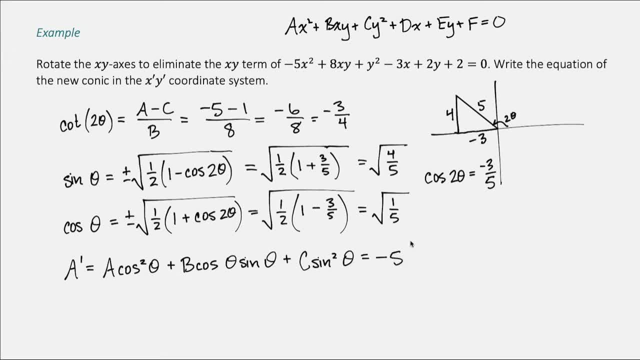 So I have negative 5.. Times, cosine of theta is the square root of 1- fifth, And then that's squared And then I have plus B, So plus 8.. Times, the cosine of theta, is root 1- fifth, And the sine of theta is the square root of 4- fifths. 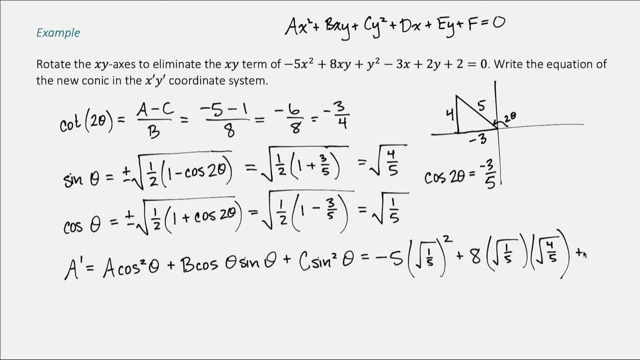 And then plus C, C is 1.. Times the sine of theta squared, So that's the square root of 4 fifths Squared. And then I can simplify this. So this is negative 5 times. This becomes just 1 fifth. 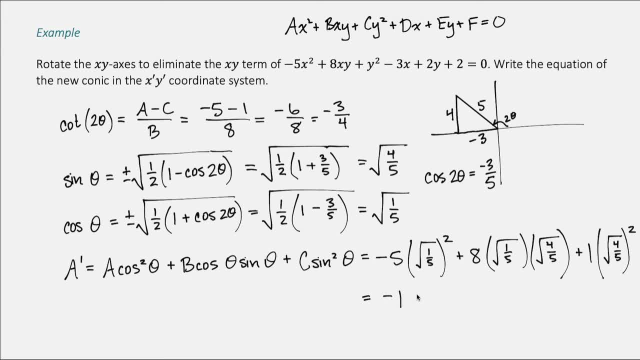 So negative 5 times 1. fifth is negative 1.. Plus, This is 8 times these two square roots, That's the square root of 4 over 25.. Which is 8 times 8 times 2, fifths. 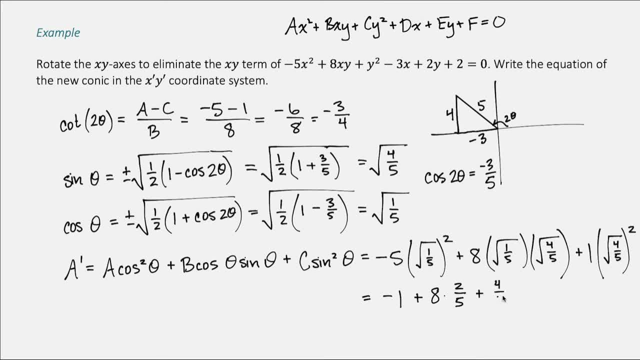 And then plus. This is 1 times just 4 fifths, Just 4 fifths. That's negative. 1 plus 16 fifths plus 4 fifths, Which is 3.. So I now have A prime equals 3.. 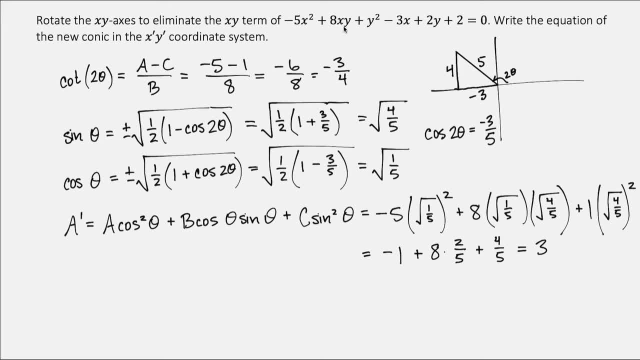 Okay, There's no B prime term Because we're eliminating the XY term, But there is a C prime. C prime is The formula: there is A Sine squared of theta Minus B Cosine theta, Sine theta. 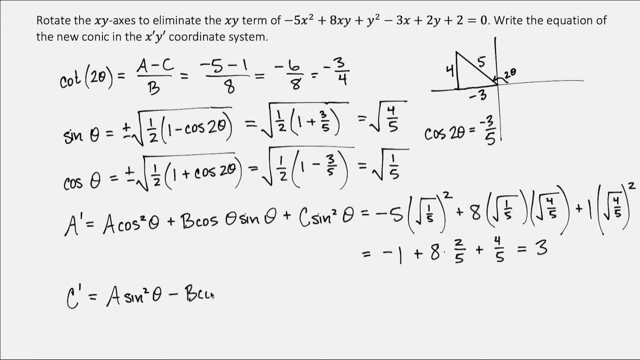 And then plus C Times the Cosine squared of theta. And so now again We plug everything in. A is negative 5. I'm going to go ahead and now skip a step While I do each of these things. So 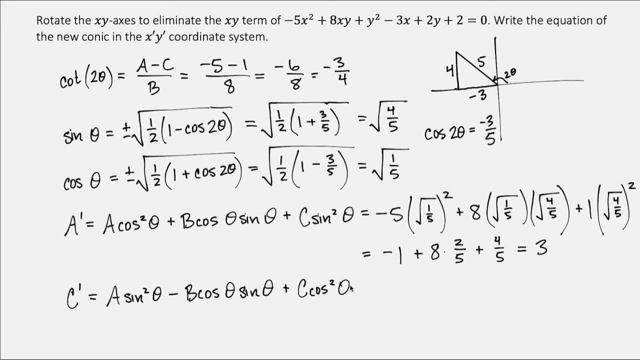 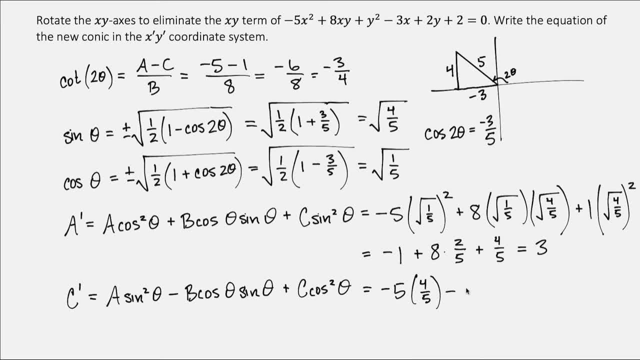 Sine, Sine, square root. So That's 4 fifths, And then Minus B is 8. Cosine Times, Sine, And multiplying these together. I did that up here And that was. 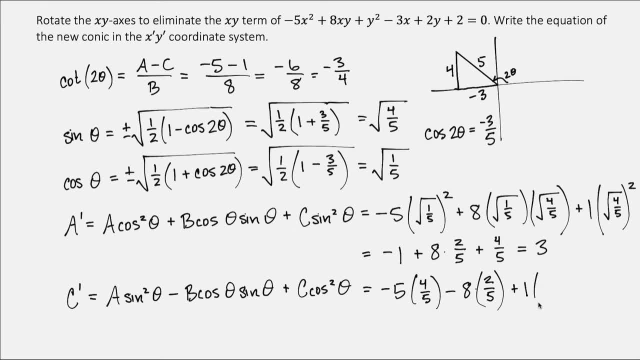 2 fifths, And then Plus C, Which is 1 times Cosine Squared, Which is Just 1 fifth minus. this is 16 fifths plus 1 fifth, And that's of course negative 4 minus 15 fifths. 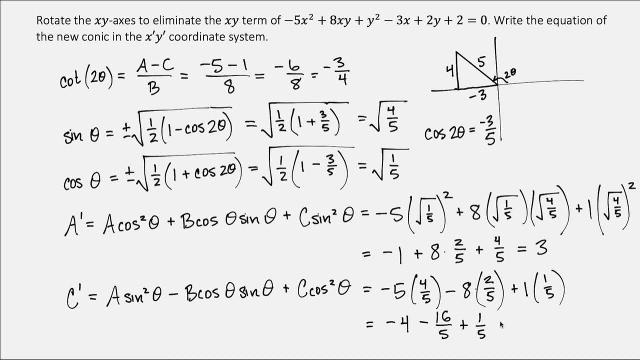 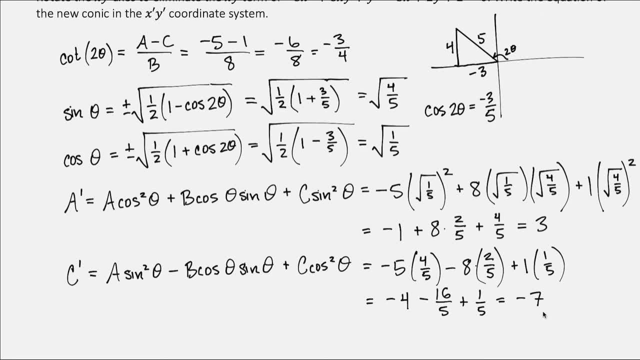 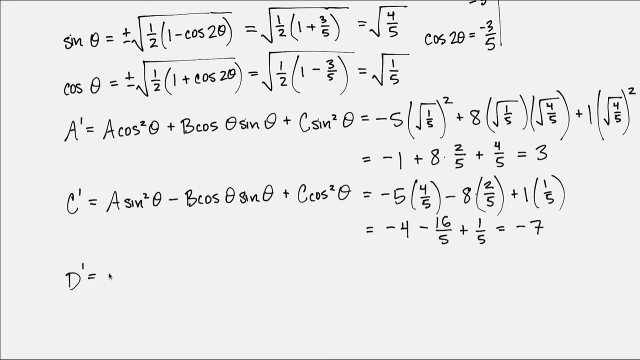 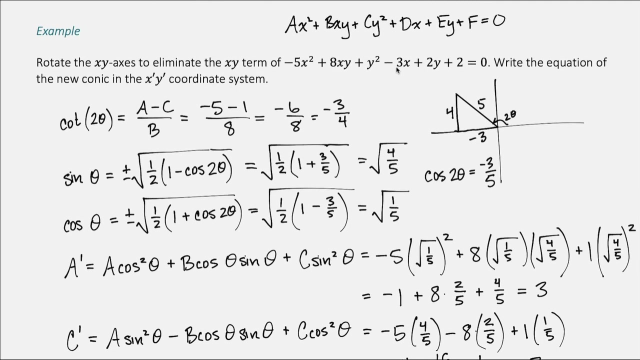 or minus 3, so that's negative, 7.. So c prime is negative, 7.. Okay, our next conversion is d prime. d prime is d times cosine of theta plus e times sine of theta. Okay, now d is up here. d is negative, 3. Negative, 3. Cosine of theta is the square root of 1. fifth, 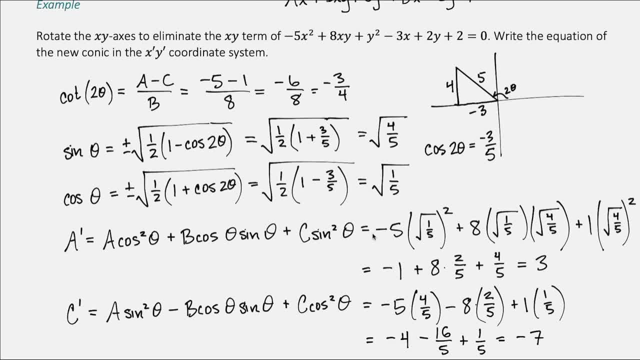 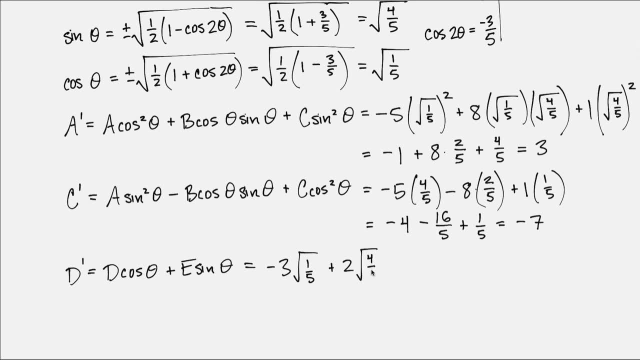 Okay, plus e, e is 2, times sine of theta, which is the square root of 4. fifths Okay, and we can of course simplify this: This is negative 3 over the square root of 5,. 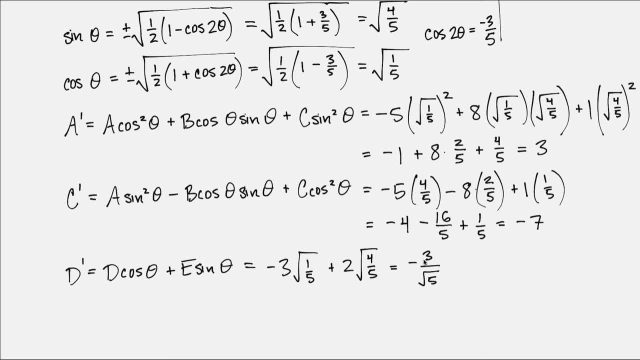 because the square root of 1 is 1, times negative 3 is negative 3.. And then plus 2 times root 4 is 2, so 2 times 2 is 4, over the square root of 5.. So this is just 1.. 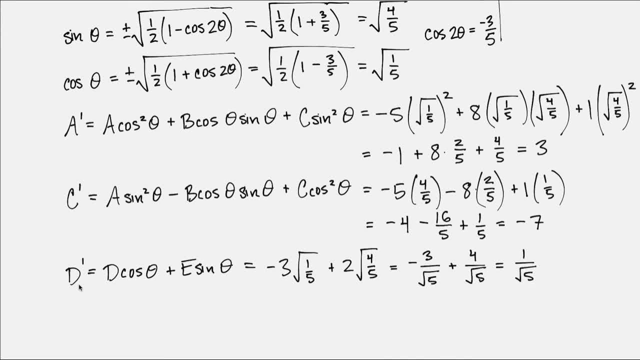 1 over root 5 for d prime And then e prime. the conversion is negative d sine of theta plus e cosine of theta, And so I got negative d, d was negative 3, so that's just 3.. Sine of theta is: 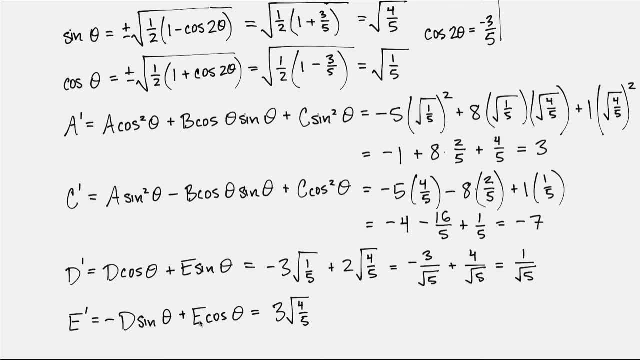 root 4, fifths, Okay, and then plus e, which is 2, and then cosine theta is root 1, fifth. And then again simplify: This is 3 times 2, is 6 over root 5, plus 2 over root 5, which is 8 over root 5.. And that's our e prime. And then 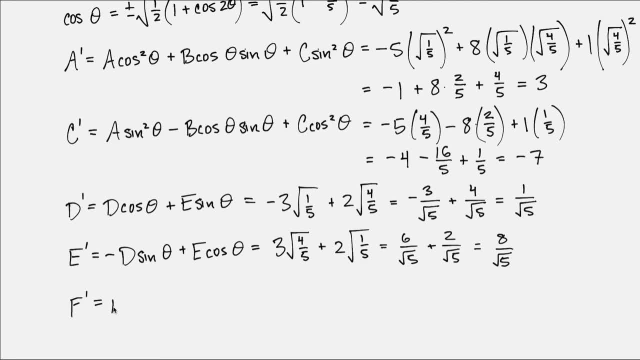 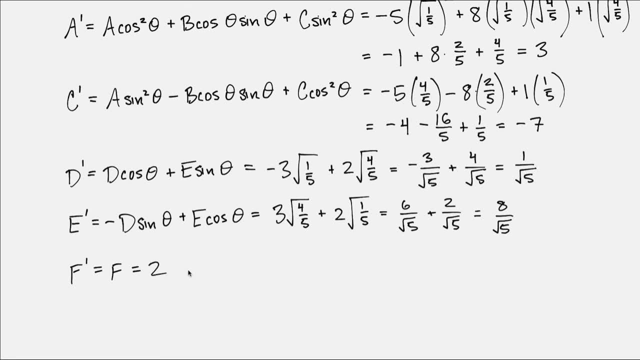 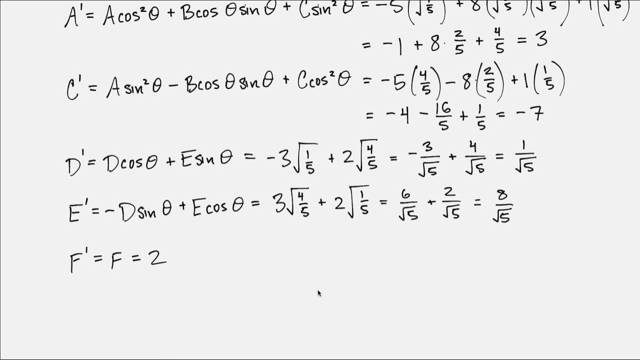 finally, of course, the easiest of all is that f prime is equal to f. There's no change there. And f here was 2, so f prime is also 2.. And so now our formula: we go through it and we just plug these things in, So we've got a prime which is 3, times x prime.